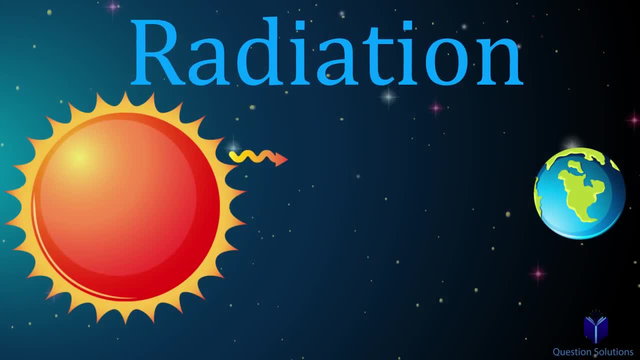 the heat sink of your computer. Lastly, we have radiation, And that's the transfer of energy because of electromagnetic waves. This transfer can happen in empty space and doesn't require any matter, But something is really hot. So, from something that's really hot to something that's 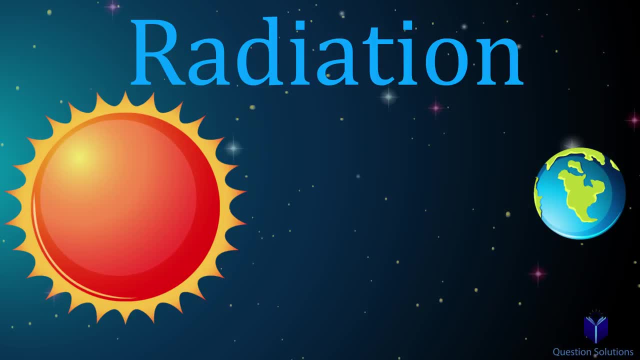 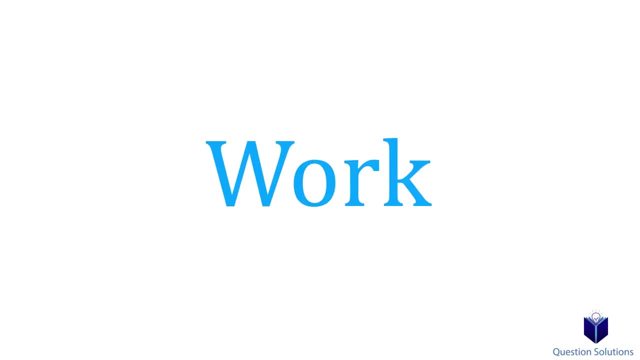 required to generate the radiation and something else is required to absorb the radiation. Now that we have a basic idea of what heat transfer is, let's talk about the second way. energy crosses the boundaries of closed systems Work. An easy way to think about it is: 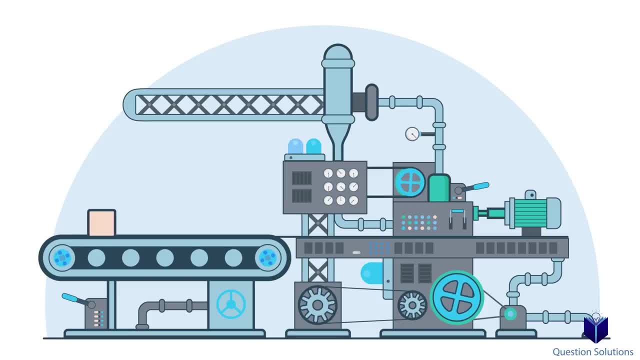 if it's not a heat transfer, then it has to be work. Work is the transfer of energy when a force acts through a distance. Examples would be work done by point forces, electrical power, such as batteries or power outlets, or even chemical work. When we look at examples, you will be able to distinguish heat and work. 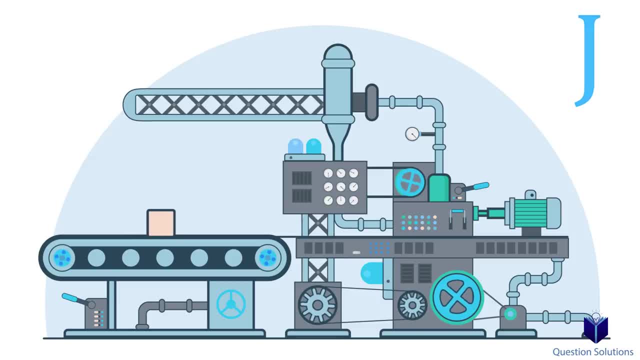 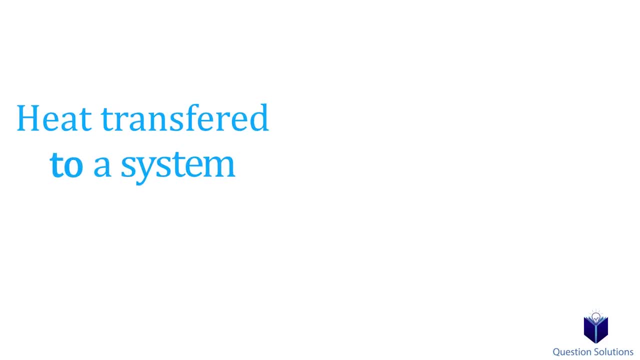 easily. The units for work is the joule. Both heat and work are directional quantities, So that means it has both a magnitude and a direction. Normally, when heat is transferred to a system and work is done by a system, it's considered positive. When heat is transferred from a system or work is done, 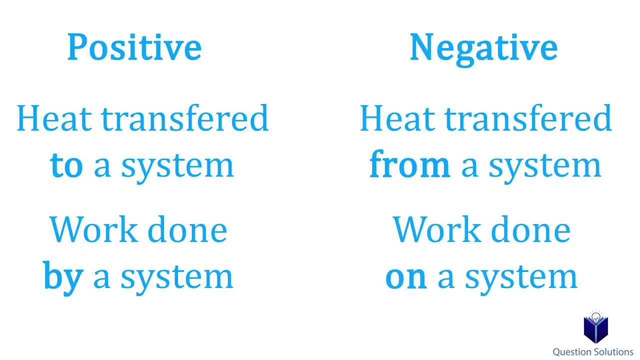 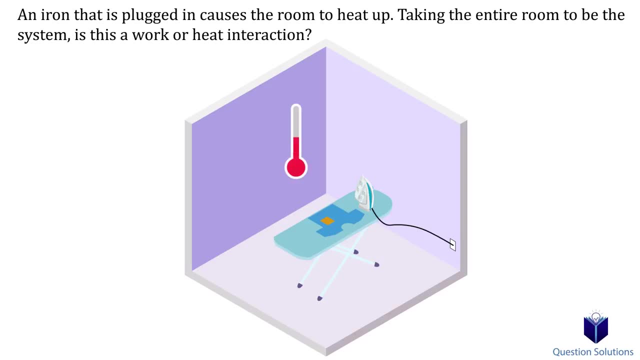 on a system, it's negative. Let's go through some examples to see if we can differentiate. Let's take a look at this problem. We have an iron turned on in a room and the room heats up, Taking the entire room, including the iron, to be the system. we need to figure out if this is a heat. 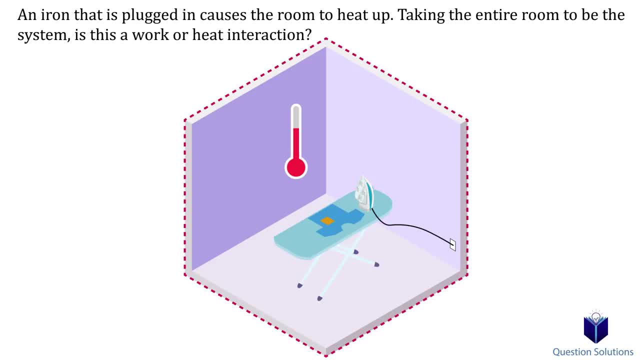 or work interaction, Since we're taking the whole room, including the iron, to be the system. the heat is caused by electrons that are crossing into the system boundary. Because of this, it's a work interaction In this question. we have an electric oven and we need to figure out the 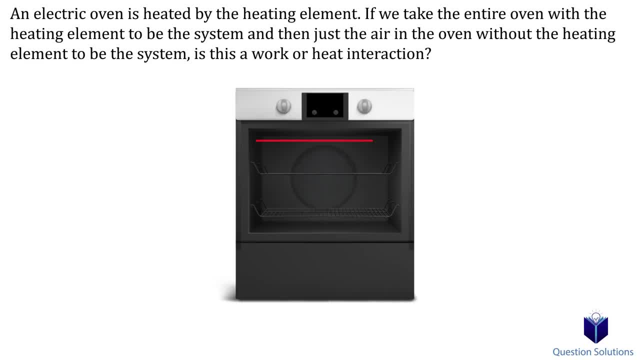 energy interaction, when we consider everything to be the system and when we consider only the air in the oven, without the heating element. For the first scenario, our boundary would look like this: Looking at the system and the surroundings, we can see that the temperature rises in the oven. 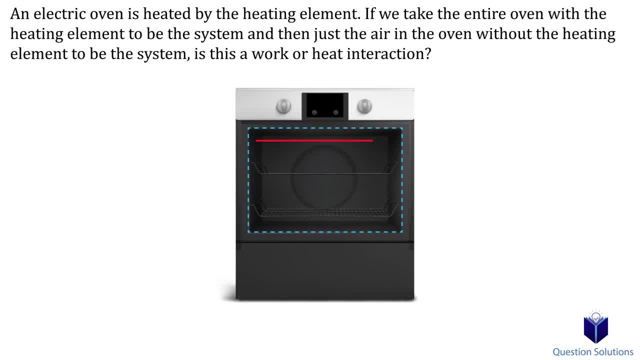 without a temperature difference between the oven and the surroundings. Keep in mind that the heating element is included in our system, So if it's not due to heat, it must be due to work. It's actually the electrons crossing the system boundary, which is